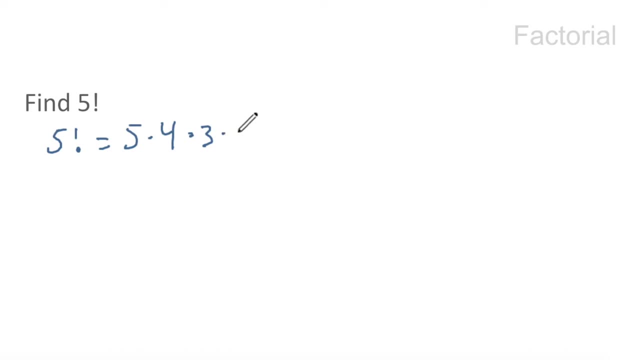 times 3.. Times 2, and we'll ignore the 1.. So when we multiply this out, 5 times 4 is 20.. Times 3 is 60.. Times 2 is 120.. So 5 factorial is 120.. Now let's figure out 6 factorial. Well, 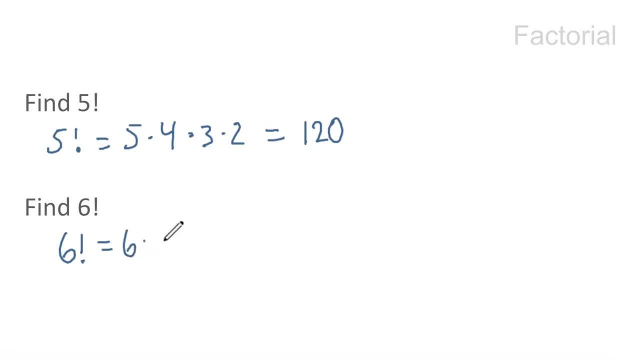 6 factorial is equal to 6 times 5 times 4 times 3 times 2,, which is the same as well. 6 factorial is equal to 6 times 5 times 4 times 3 times 2,, which is the same as well. 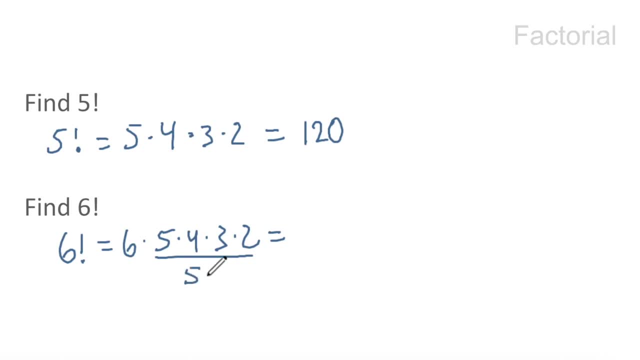 see this: here is 5 factorial right. So it's really 6 times 5 factorial. 6 times 5 factorial, So this is 5 factorial right here. So 6 times 5 factorial is 6 times 120.. 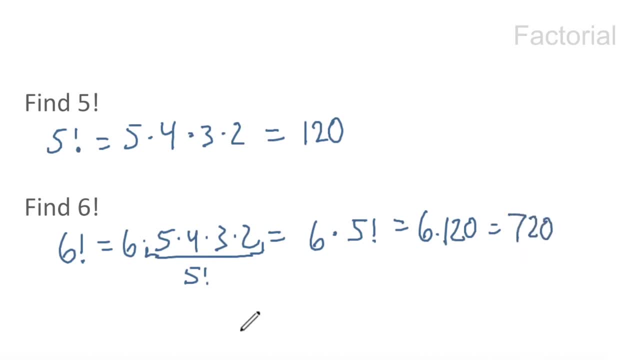 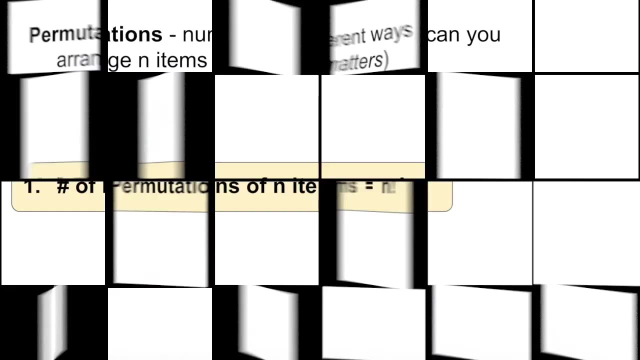 And that is equal to 720.. So it's pretty easy to calculate factorials. It's really just adding more numbers out in front and multiplying them out. Now let's see how we can use factorials to solve problems. Permutations are the number. 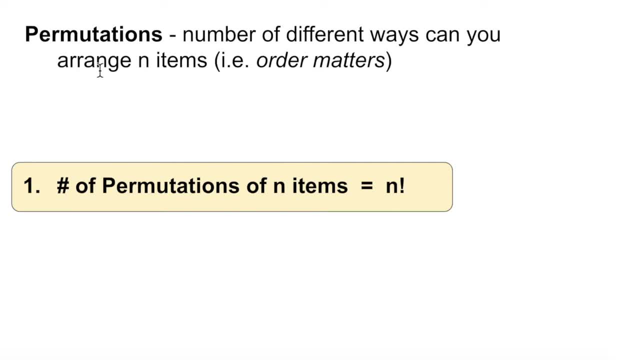 of different ways you can arrange in items And order matters. You'll see what this means in a second. So the first rule here, the first formula we're going to learn, is the number of permutations of in items is equal to in factorial. That's a really easy equation. 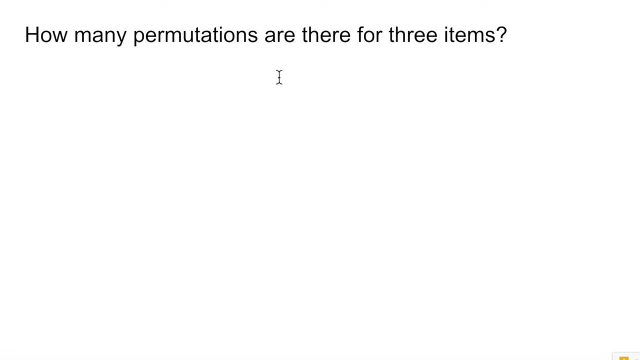 isn't it? So how many permutations are there for three items? Gee, this should be a piece of cake. Three items. the number of permutations for three items is just equal to 3 factorial, isn't it, Which is 3 times 2.. Again, we can ignore the 1., And that is 6.. Wow, that was. 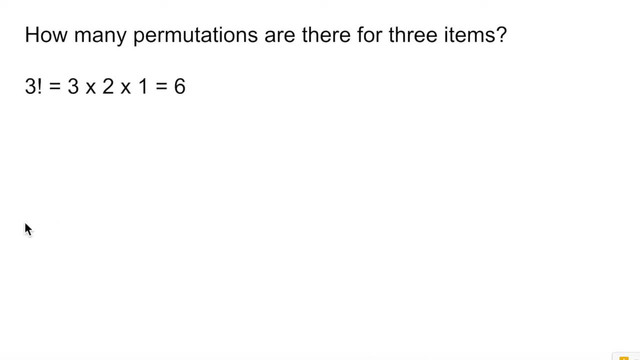 really simple. So 3 times 2 times 1 equals 6.. And if you want to see that visually, you can also look at the formula. Now let's say we have a permutation of a- b, c. We have a permutation of a- b, c And. 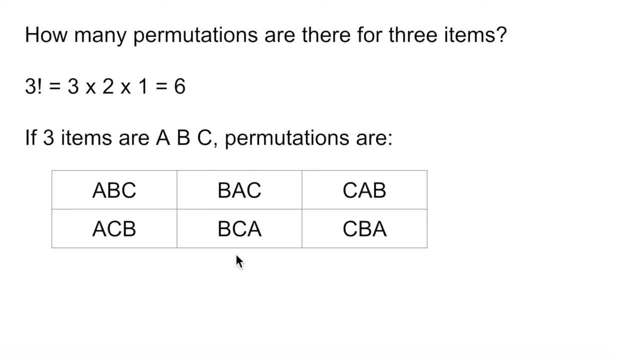 if we look at the formula visually here, let's say our three items are a, b and c, The six different permutations of a b c. these three items are: a b c. a c, b, b. a, c, b c. 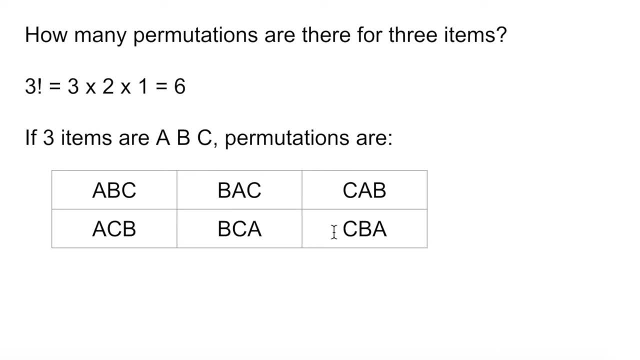 a, c a b and c b a. So what do we mean when we say that order matters? Well, look, we have the same three items in, actually, all six of these different permutations, but they're all the same. So if order didn't matter, these would all be the same thing. But since order 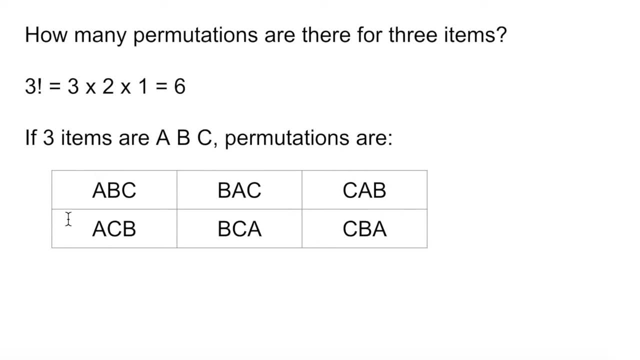 does matter. we've got the same six items arranged in six different orders, So we count this as six different permutations. So a permutation is an arrangement in order of items in a different order, And the items needn't necessarily be letters. Here we use just letters as an. 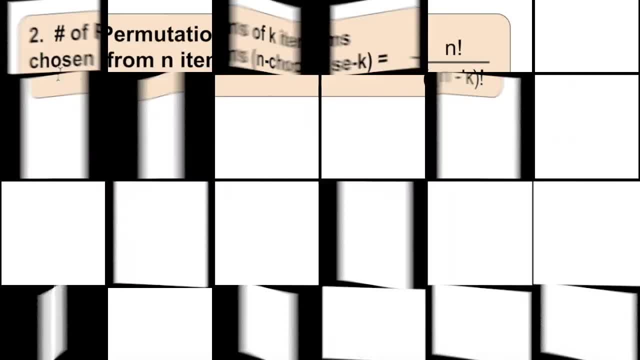 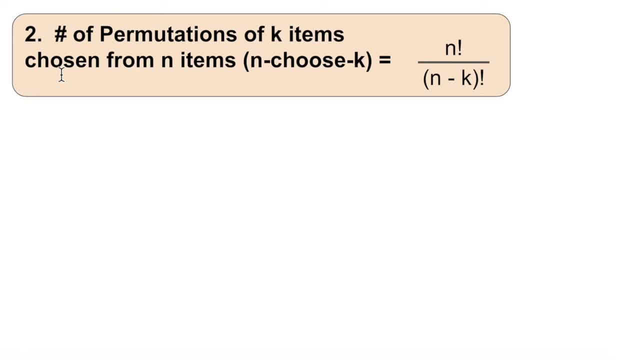 example, but they could be anything really. So our second formula here is the number of permutations of k items chosen from a set of n items. This is an n choose k permutations problem, because we want to know the number of permutations of k items chosen from a set. 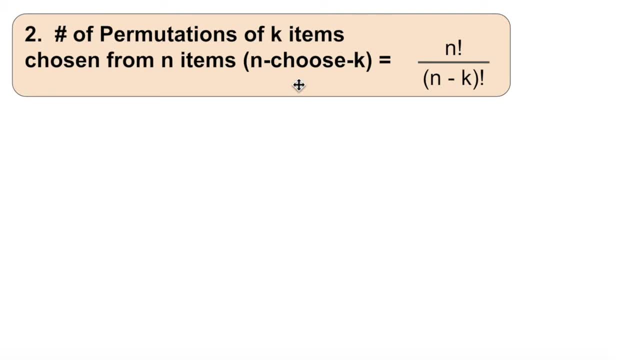 of n items. For example, if we have a box of ten toys and we choose six of those toys, how many different orders of items are there? Well, let's see n- factorial over n minus k in parentheses: factorial. So let's use that to solve some problems. How many permutations are there to choose? 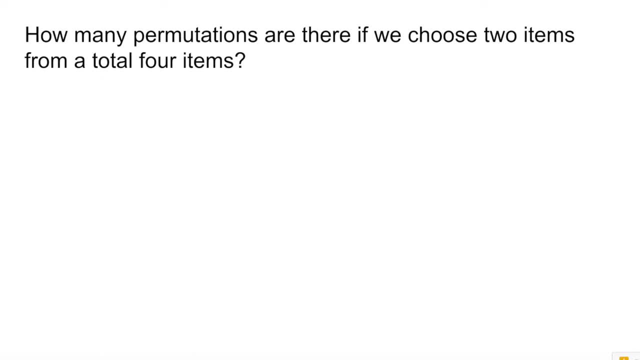 two items from a total of four items. Well, all we have to do is apply that formula we just learned. So the number of permutations of- let's see what is n here. n is equal to four, right? Because there are four items, There are a total of four items, So n is equal. 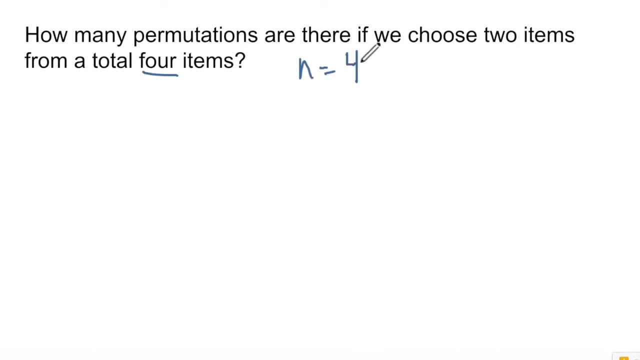 to four. That's the number of items. K is the number of items we're going to choose, and we're going to choose two items, so k is equal to 2.. Now we just need to plug that into our formula. Our formula was: the number of permutations is equal to n factorial over n minus k. 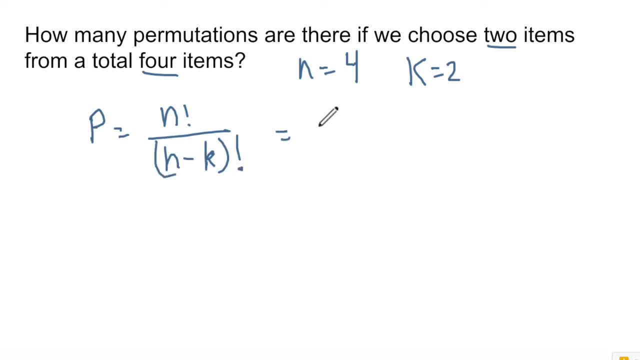 factorial, and that's equal to 4 factorial. or we can write it out as: 4 times 3 times 2 times 1, divided by n minus k. well, that's 4 minus 2, right, that's right. 4 minus 2 factorial. so 4 minus 2 is 2, so this is really just 2. 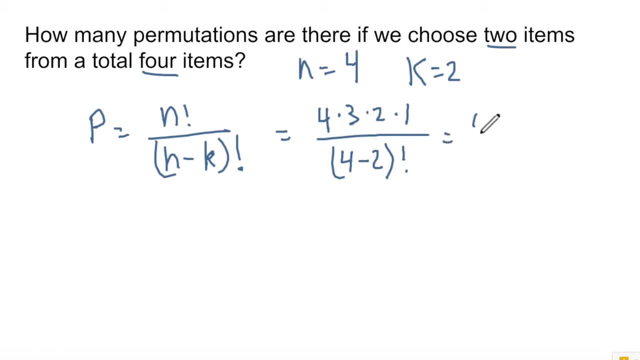 times 1. down on the bottom, isn't it? let's write that out: 4 times 3 times 2. ignore that. one divided by this is 2 factorial, which is just just 2. really, 2 factorial is just 2. so that's our answer. here. the 2s cancel each other out and we just get 12, so that is 12. so. 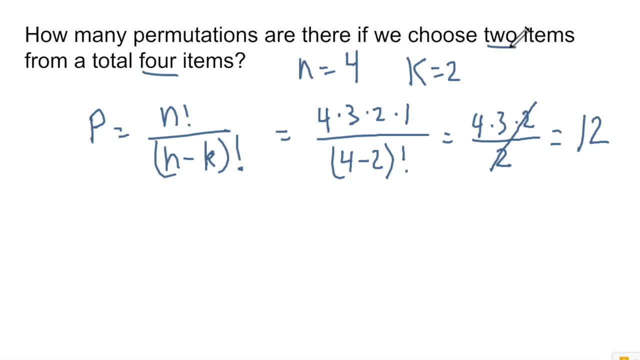 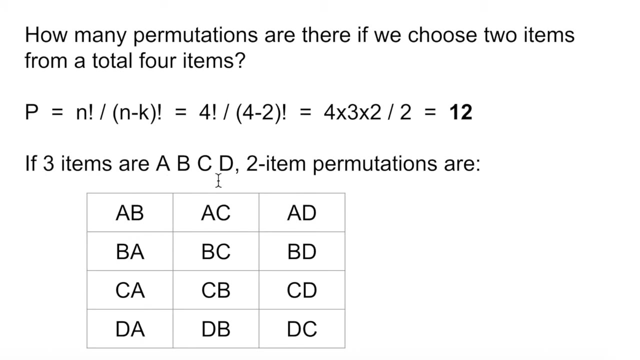 the number of permutations if we choose two items from a set of four items is 12. there are 12 possible permutations and if you need to see that visually here, look if our items are abc and d and we have to choose two items, these are all the different. 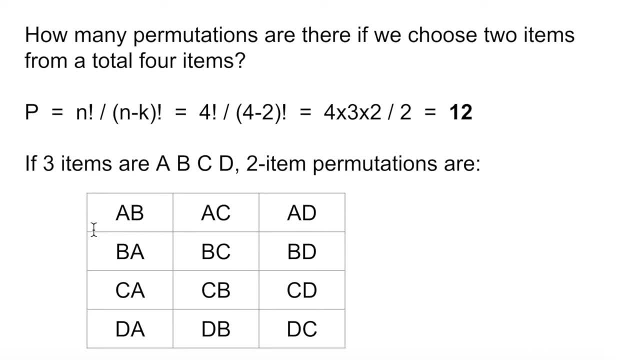 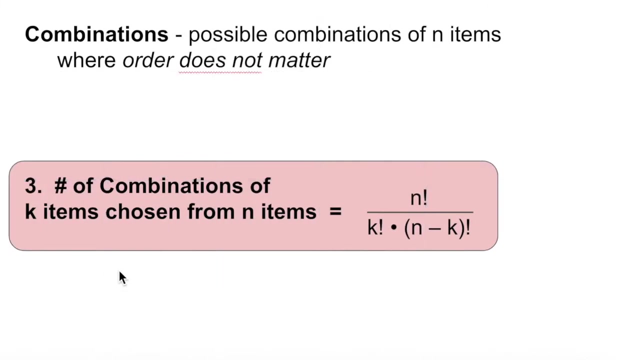 possible permutations of of those four letters, so AB and of course, BA. again, order matters, right, so different order, same two items. these account is two separate permutations, CA and then, of course, AC. so these are our 12 possible permutations for those four items, And our third and final formula here that we're going to learn in this video is a number. 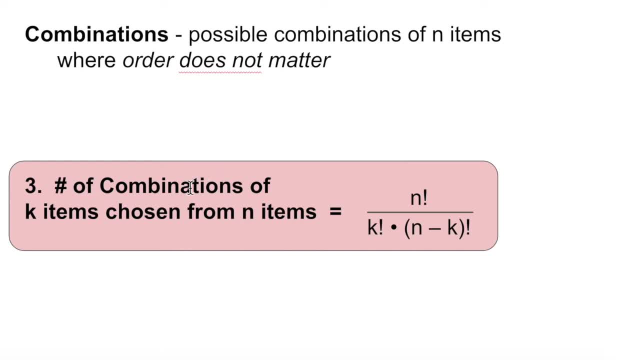 of possible combinations of n items, where order does not matter, And the formula for that is exactly the same as formula number two, except that what we did is we added a k factorial in the denominator. So this is also n choose k. but this is combinations, not permutations. 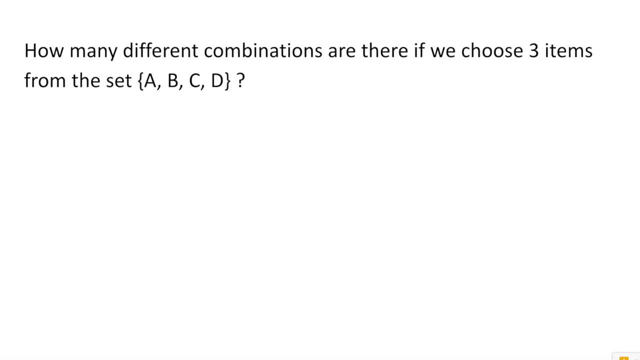 Let's take a look at a sample problem for combinations using this formula we just learned. So how many different combinations are there if we choose three items from the set ABCD? So here we have four items, right? So n is equal to four. 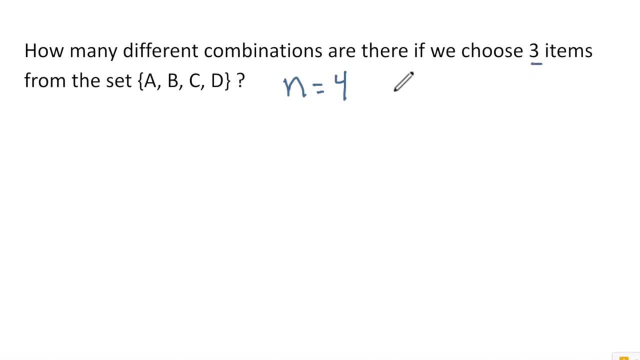 And how many items are we going to choose? Well, we're going to choose three, right, So k is equal to three. So our formula is: combinations is equal to n factorial over k factorial. Okay, Okay, So k factorial times n minus k factorial. 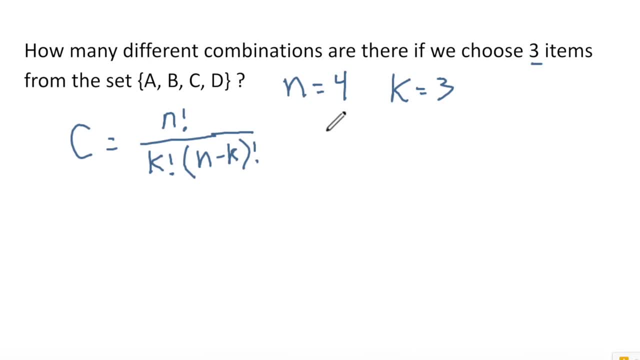 So that's our formula. Now we can just plug in three and four for n and k And we're going to get, let's see, four factorial, which. let's multiply this out Four times three times two, And sometimes it helps to write it out as four times three times two, because you can cancel. 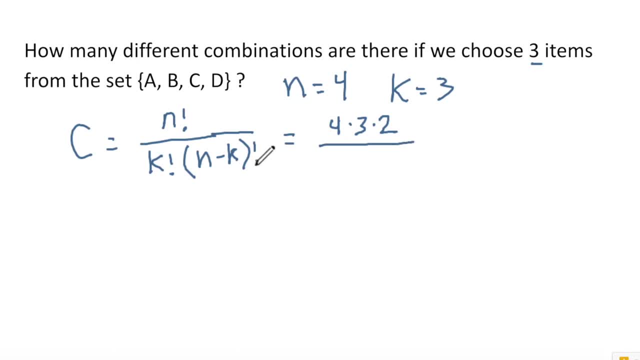 out a lot of stuff in the numerator and denominator. It makes the math a little easier at the end. K factorial. K factorial is three times two, right, That's three factorials, That's three times two. And then n minus k is four minus three. 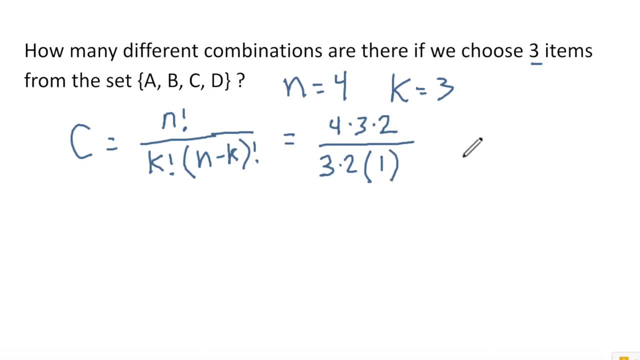 Well, that's just one, isn't it? So that's what we get for n factorial over k factorial times, n minus k factorial. So there are this many combinations. And look the three and the two. that three cancels out with this three and this two cancels. 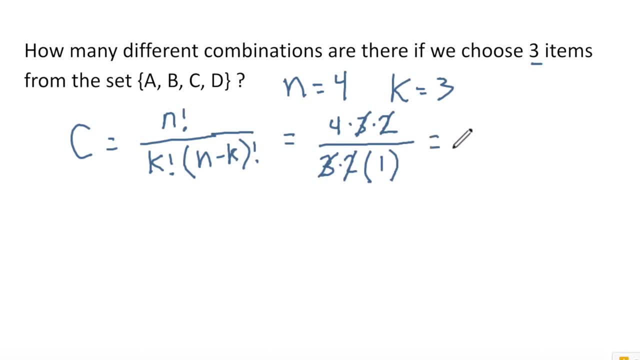 out with this two. So what we get is just four over one, Which is simply four. So there are four different combinations, So this whole thing just reduces to four. Then you see why I write them out like this. You can write it as four factorial, and then you can do the long map and then reduce your 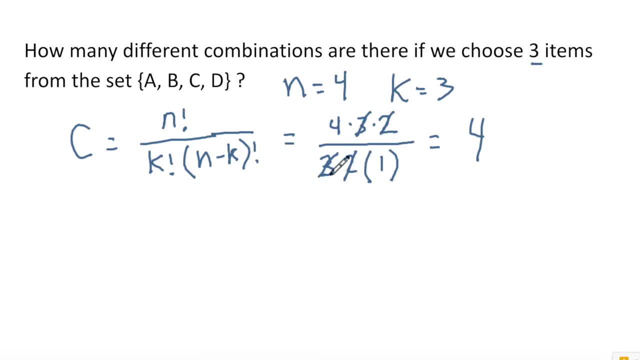 fraction. That's just a little more work. It's easier to just reduce stuff after you write the problem out like this. So here are the actual combinations: abc, abd, acd and bcd, Srb, srb, Spear. 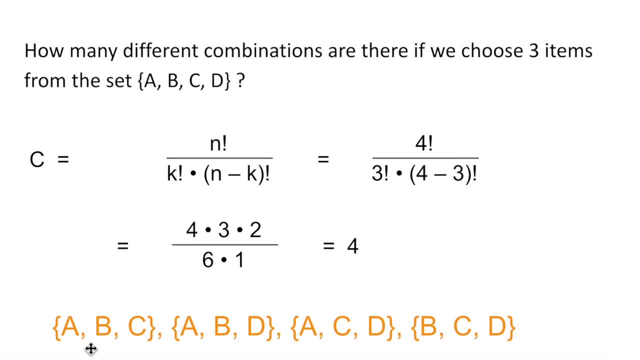 So we don't get to write B A, C, B, C, A. We don't get to write all these same items different order, because those would be permutations. These are combinations. Each of these is a unique set of items. 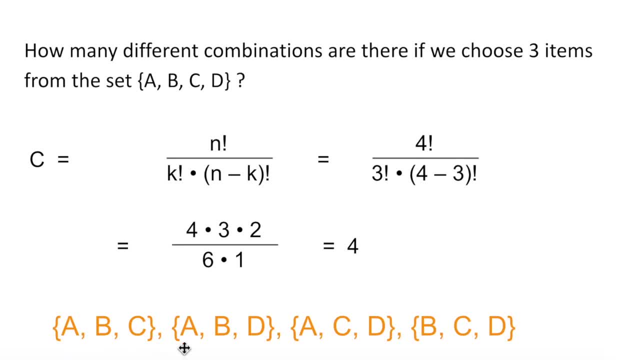 So those are the three formulas. You realize, when you're looking for combinations where order doesn't matter, you just add this K factorial on the bottom and that gives us combinations where order doesn't matter. If order does matter, you just scratch that K factorial off the bottom. 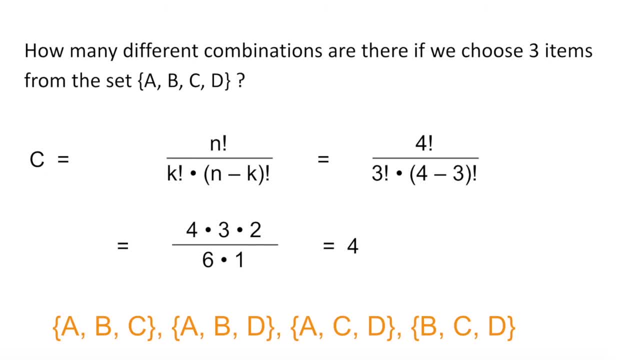 So there are two different types of in-choose-K problem. What you need to figure out when you're looking at a problem is whether or not order makes a difference in the question they're asking you. So to summarize here, these are the three formulas that we've covered. 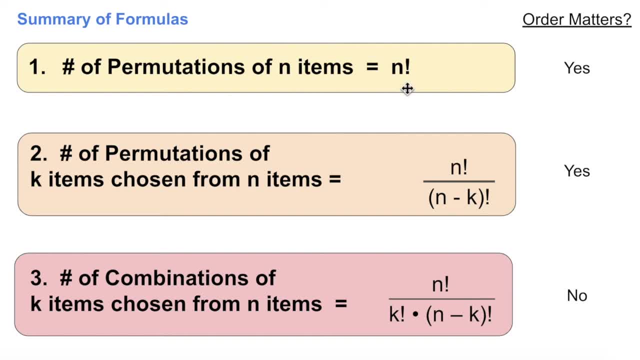 Number one is the number of permutations of in-items. We're not doing any choosing here, so there is no K, There's the number of permutations of in-items. Does order matter? Yes, Two is the number of permutations of K items chosen from a set of in-items. 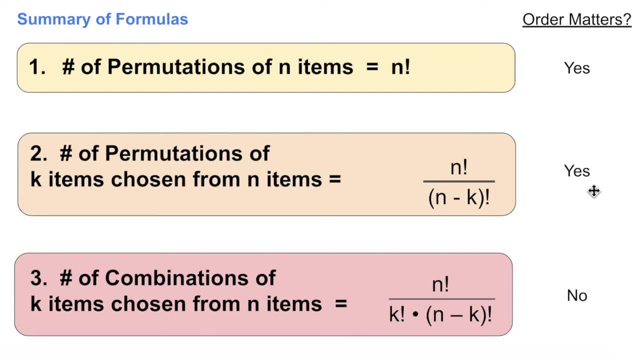 And that's N factorial over N minus K factorial. And again, order does matter because these are both permutations, number one and two. Number three is combinations, where order does not matter. So the difference in the formula here is that we added the K factorial on the bottom. 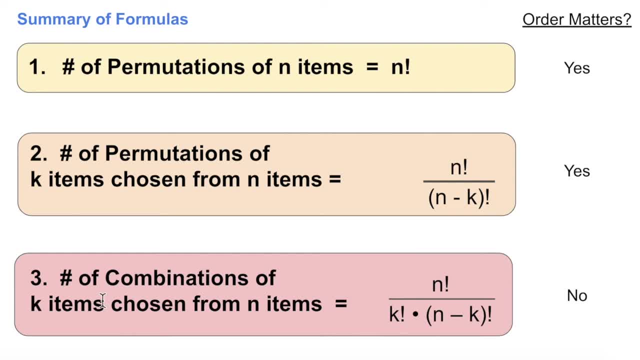 because order does not matter. So those are our three formulas. Now, when we see a problem, we just need to determine which one of these to use. It's going to be easy to rule out number one if we're given a K or we're not given a K. 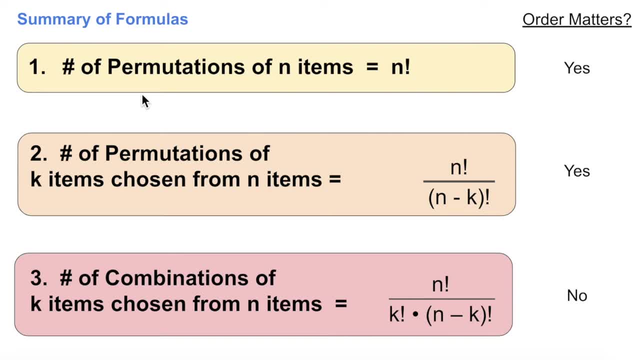 So if we're just given a number of items and asked how many different combinations or permutations or it doesn't matter what to call it, if you're only given a number of items and you're not choosing any of those items, then pretty much all we can calculate is N factorial. 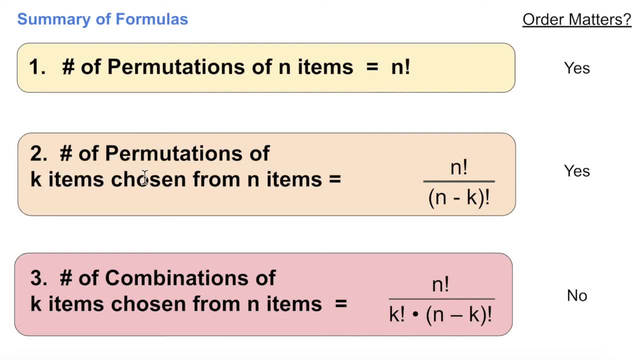 If we're choosing, If we're choosing, If we're choosing a subset of a given set of items- in other words, there's both an N and a K given in the problem- then we just need to figure out if they want us to count the same items in different orders as two separate permutations. 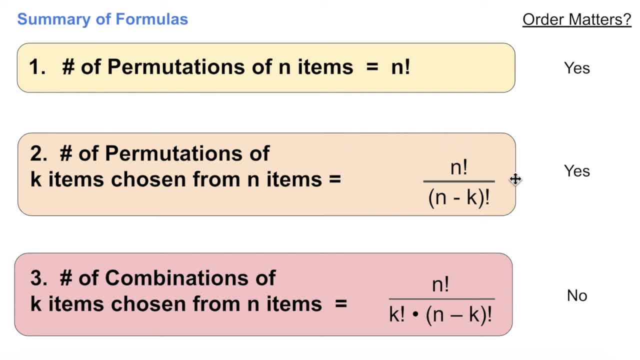 And if they count that as two separate entries, then that is this equation, And if you don't double count those, then we're looking for combinations number three. So three formulas, not that complicated, But let's go ahead and apply those to try and solve about three or four problems here. 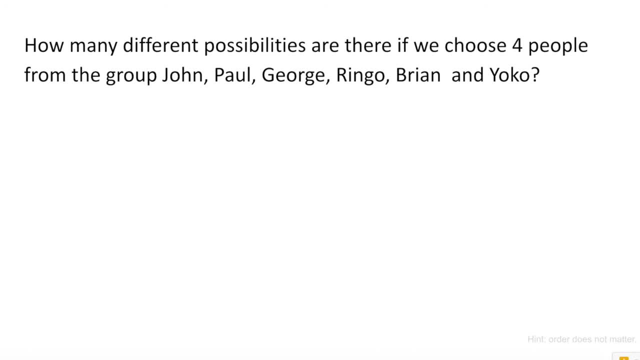 First one: how many different possibilities are there? We'll just call it possibilities. We have to decide whether this is combinations or permutations. If we choose four people from group John, Paul, George, Ringo, Brian and Yoko- Hmm, how many names do we have here? first, 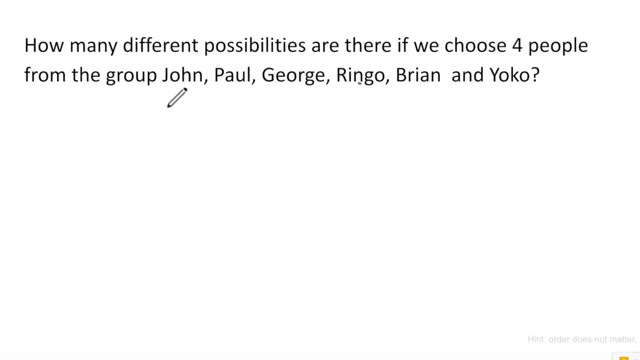 One, two, three, four, five, six. It looks like we have six names. So N is the number of names in that set, which is six. And then it says we're going to choose four. So K is equal to the number we're going to choose, which is four. 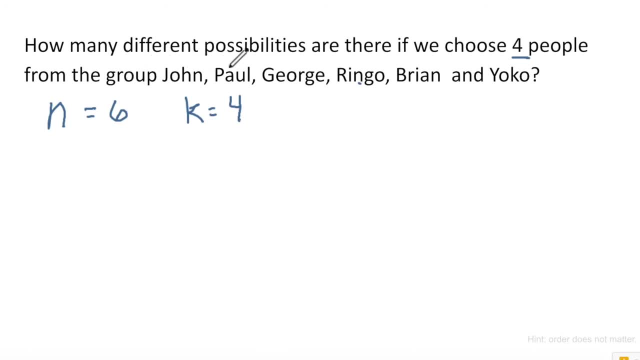 That's our subset. And then they're asking us: how many different possibilities are there? Well, does order matter? In other words, is John Paul, George and Ringo the same as John Paul, Ringo and George? 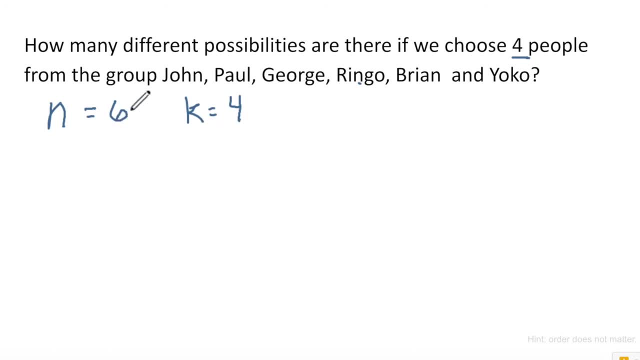 Yeah, they're the same. Order doesn't matter. We're not lining people up, We're just choosing subsets. So since order does not matter, let's see. We want the combinations, one which is N factorial over K factorial times N minus K factorial. 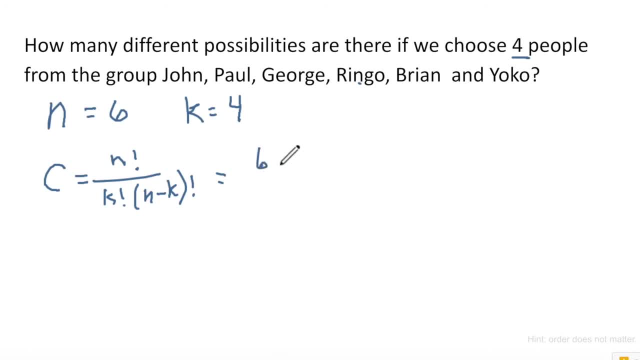 And that is equal to six factorial. I'll write this out: Six times five times four times three times two, divided by K factorial, which is four, Let's see Four times three times two, And then N minus K factorial is six minus four. 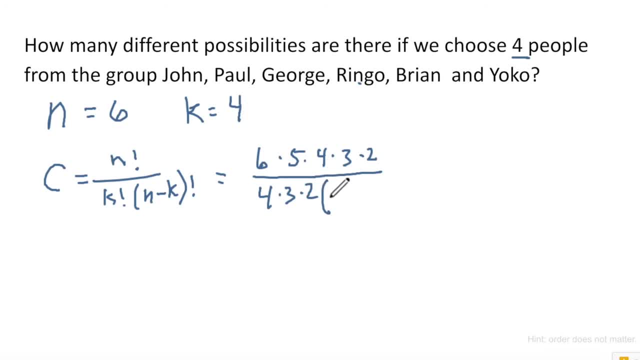 So that's two factorial. right, You have six minus four. So that's two factorial in here, And two factorial is just two. So that is it. Our N minus K factorial is just two. So now we can do some cancellation before we do any multiplying. 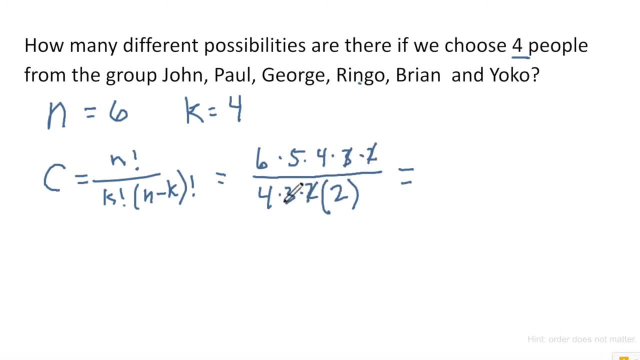 So we can cancel out this two and this two, this three and this three, this four and this four, And what we get is six times five divided by two, Divided by two, That's 30 over two, And that gives us 15.. 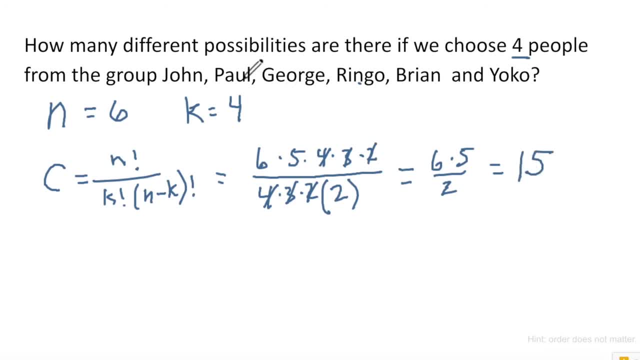 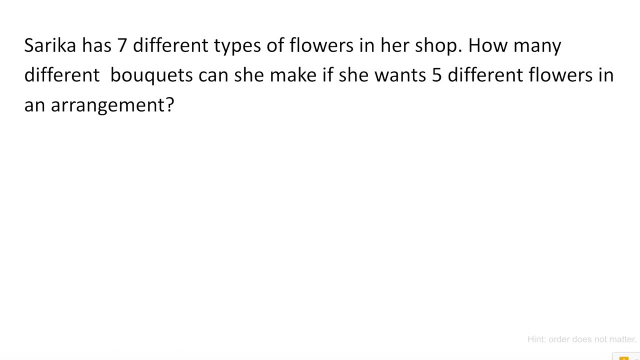 So 15 different possibilities, or 15 different combinations of four names chosen from this set of six names. Let us try another problem. Sarika has seven different types of flowers in her shop. How many different bouquets can she make if she wants five different flowers in an arrangement? 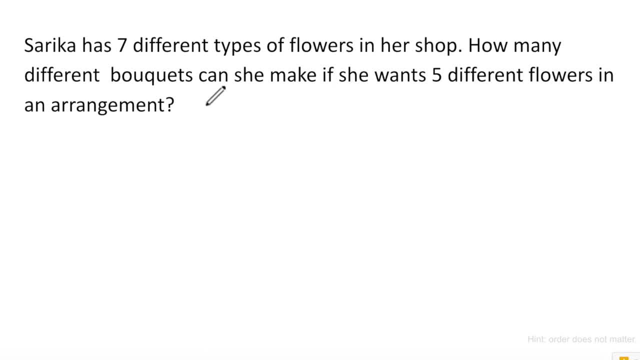 Well, okay, Let's first figure out what N is. N is the total number of items in the set, And in this case an item is a different species of flower And she has. it looks like seven, So N is seven. 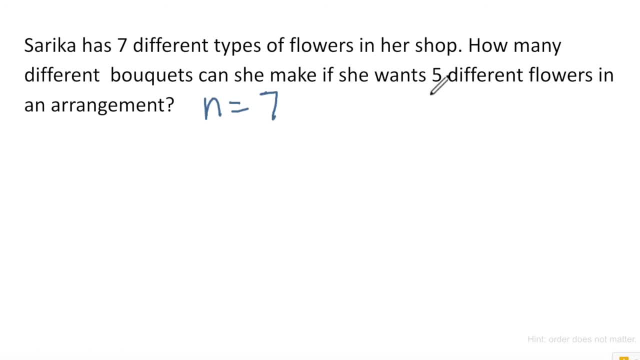 And then how many is she going to choose for each bouquet? Well, it looks like five, So the number she chooses is called K. That's our variable K. K is equal to five, So we have N and K. We need to decide whether or not order matters here. 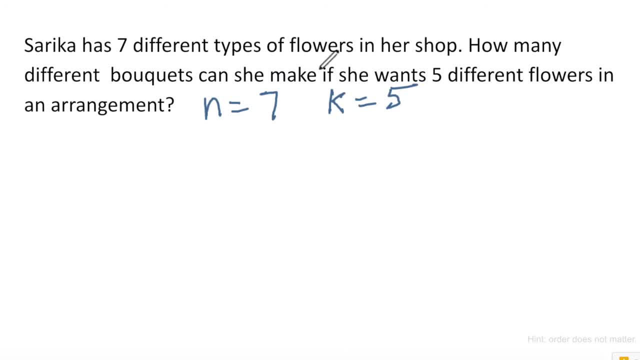 She's arranging flowers in a bouquet Order does not matter. What we're going to do is find out what combinations is equal to N factorial over K factorial times, N minus K factorial, And we just plug in our numbers, calculate this. So let's see. 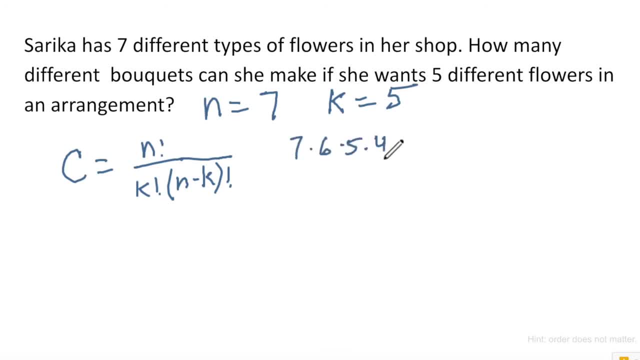 Here we get seven times six times five times four times three times two. Divided by K, factorial is five times four times three times two. So all of this is going to cancel out. All of this is going to cancel out, isn't it? 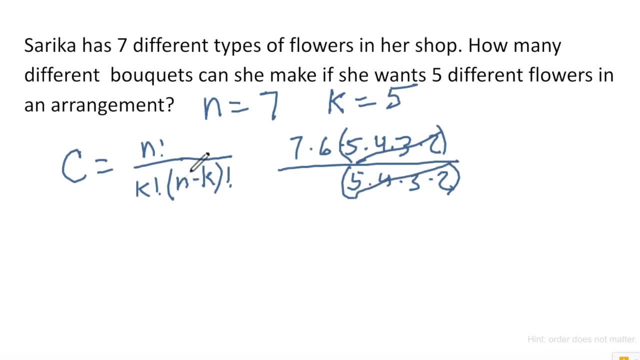 Scratch that, Scratch that. And then we still on the bottom need to write N minus K factorial, which is seven minus five factorial. So seven minus five, Seven minus five Factorial, And that is two, That's two factorial. 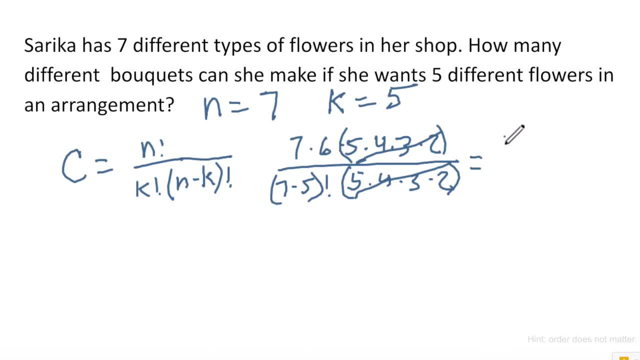 So what we get again is pretty simple here: Seven times six is forty-two over two And that is twenty-one. So our answer here is twenty-one. That whole thing works out to twenty-one different flower arrangements. Let's try another one. 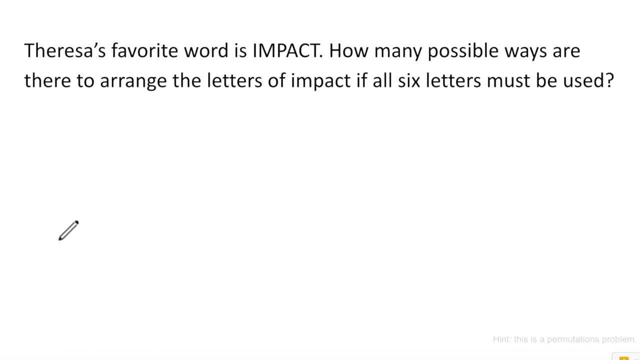 Theresa's favorite word is impact. I don't know why. That's kind of weird, but whatever, How many possible ways are there to arrange the letters of impact? if all six letters must be used? Hmm, Is she choosing a subset of those letters? 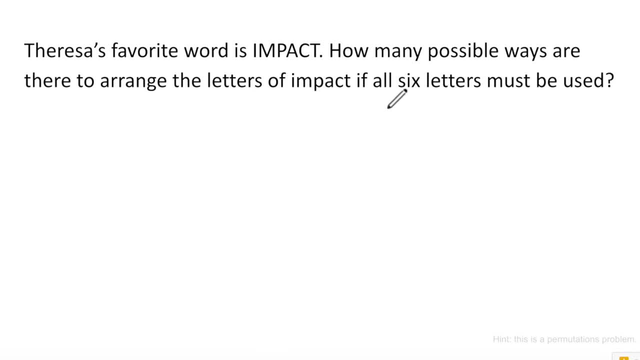 No. Is there any value given for K? No. So all we're given is a six-letter word and we want to know how many different possible ways there are to arrange. That should be a clue, this keyword here: arrange those letters. 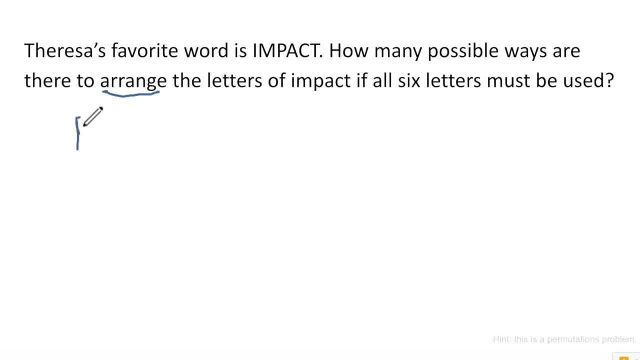 So this is just in factorial. This is permutations. We're looking for permutations of six-letter word and that's going to be equal to six factorial. So that is equal to six times five times four times three times two, And we actually already did this earlier in the presentation here. 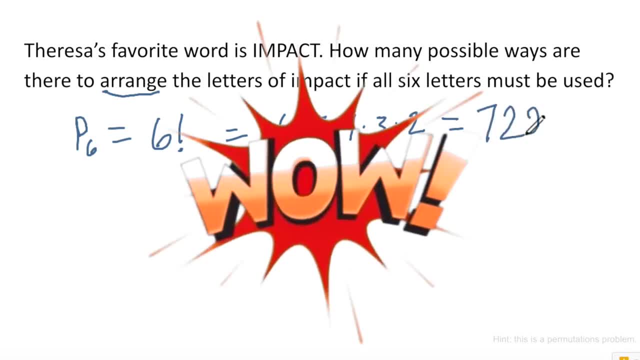 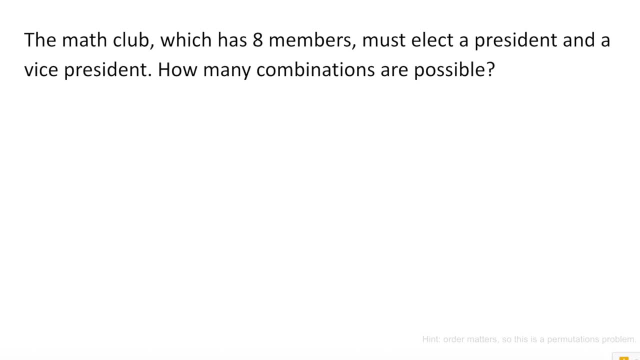 That multiplies out to seven hundred and twenty. So that one was pretty easy. And our final problem here: The math club, which has eight members, must elect a president and a vice president. How many combinations are possible? Hmm, Okay. 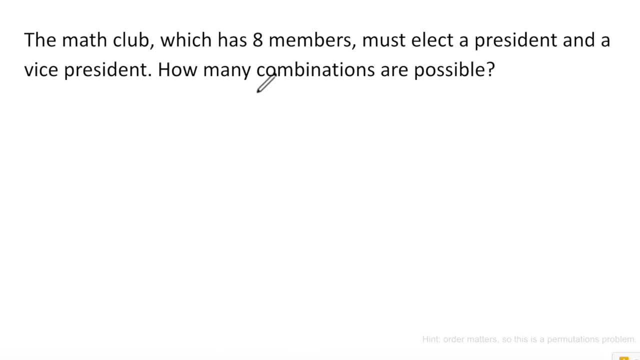 They call it combinations, but that doesn't necessarily mean that it's combinations. So let's see. First let's figure out what N is. N is equal to the number of members. here We have a total of seven. We have a subset of eight people. 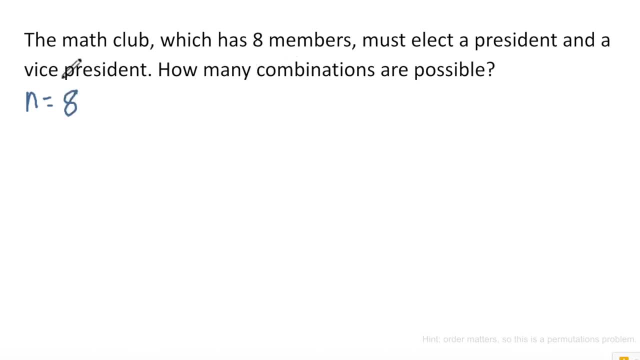 So N is eight, K is. let's see, there's a president and a vice president. so I'm going to say K is two. Our subset size is two. Next thing we need to determine: does order matter? Well, if Bob is president and Jenny is vice president, that's not the same thing as Jenny is president and Bob is vice president. 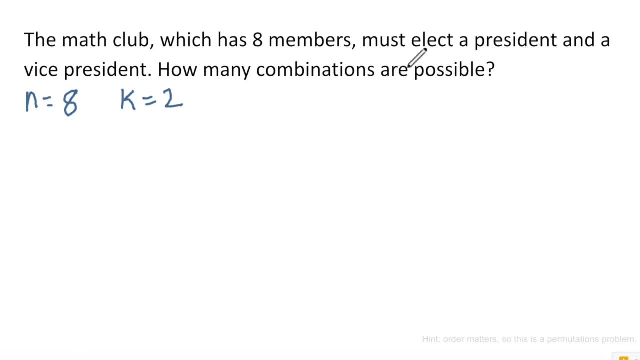 So in this case, order does matter. So what we're looking for is permutations, not combinations, right, Because these are two different positions. If we were just selecting two board members, maybe we would use the combinations formula, But in this case we have a president and a vice president, which are two different positions in the organization. 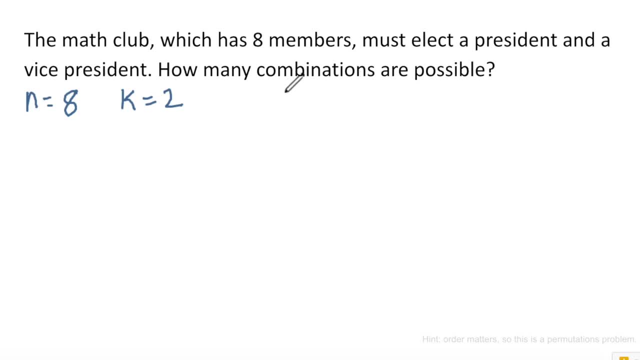 So we want to know how many different combinations are possible. What we're really looking for is permutations. So let's figure out the formula here for permutations. Let's see That's N factorial over N minus K factorial, And that is equal to eight factorial, or eight times seven times six times five times, four times, three times two.